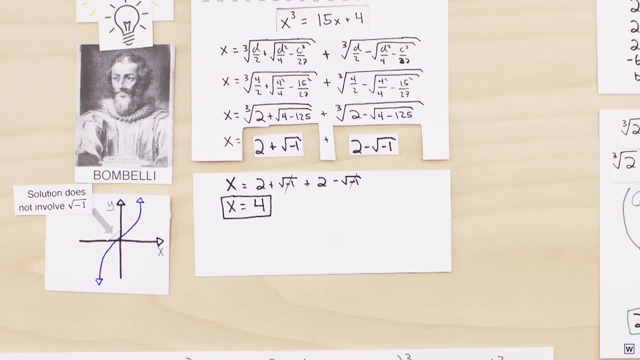 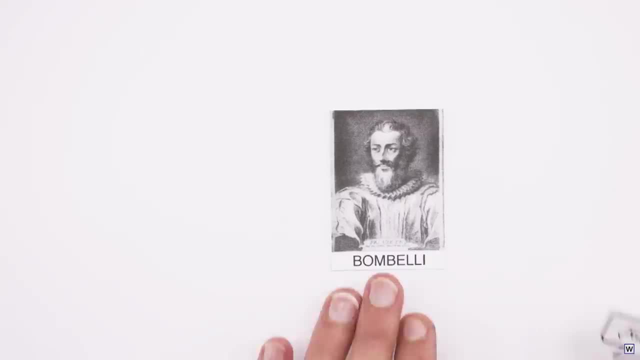 We left off with Bombelli's discovery that if he allowed the square root of minus one to be its own number, he could solve problems that had been stumping mathematicians for decades. Despite the usefulness of his discovery, Bombelli and other mathematicians generally 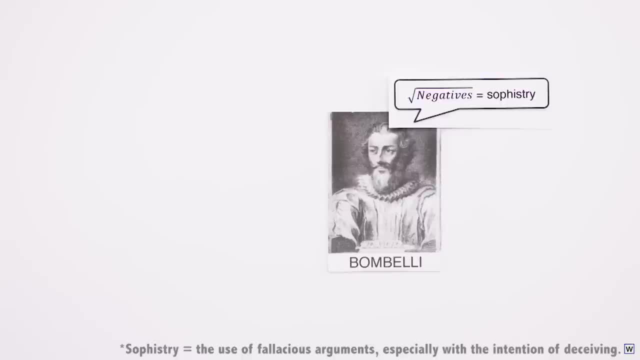 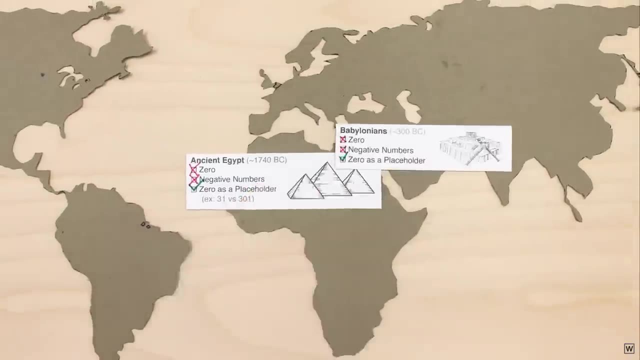 regarded it as a hack. After all, what could it possibly mean to take the square root of a negative number, Just like our friends zero and negative numbers? before, the square root of negative one was generally regarded with suspicion because it didn't correspond to. 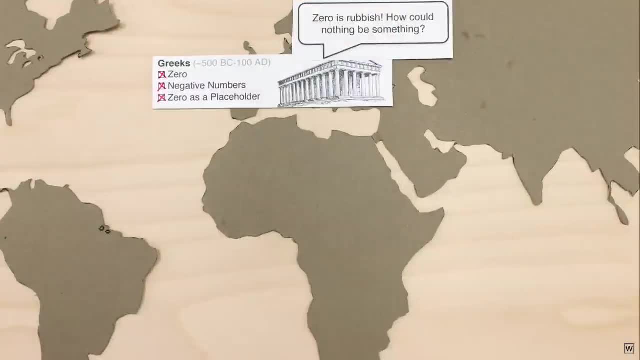 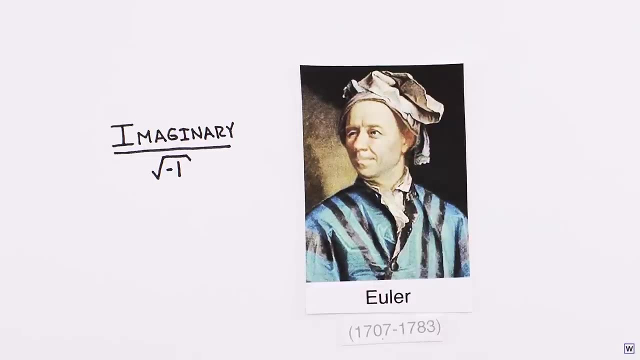 anything people could think of in the real world. For this reason, the square root of minus one was given the terrible names imaginary or impossible. A century or so later, Euler began using the symbol i to indicate the square root of negative one, making the algebra less. 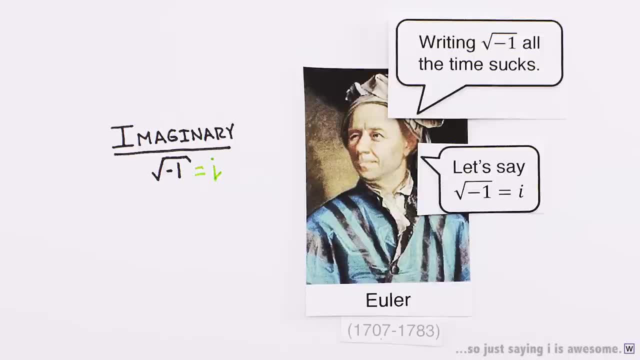 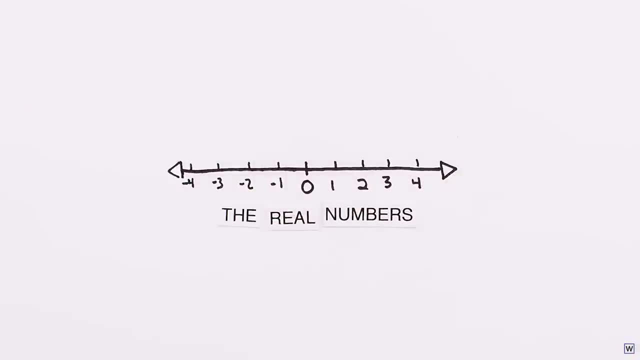 clunky. Unfortunately, the name imaginary stuck around, and that's still what we call these numbers today. In response, everything on the original number line gets the name real. When we put together a real and an imaginary number, we obtain what we today call a complex 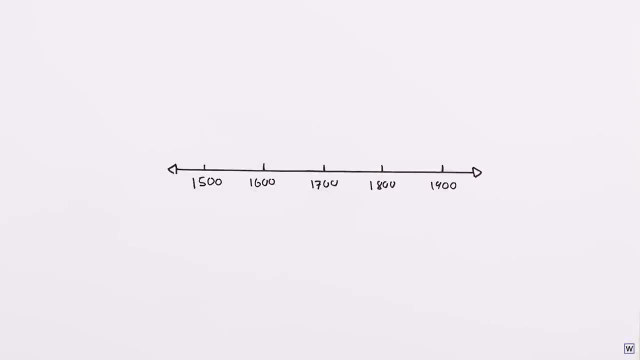 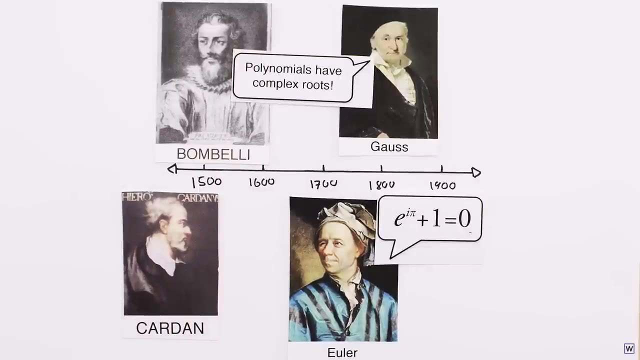 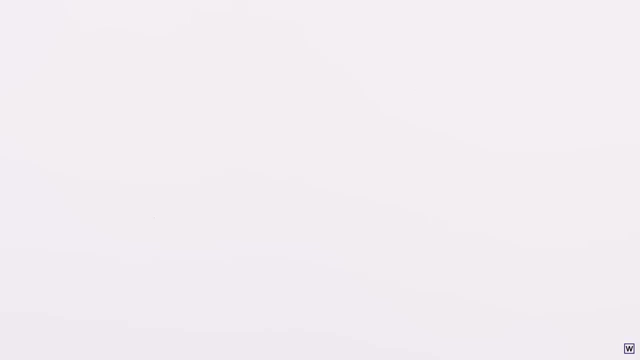 number. What is remarkable about this time period is that, although imaginary and complex numbers were used in calculations and derivations, the deeper meaning behind these numbers was left undiscovered for over 200 years after Bombelli's death. Before we dive into this deeper meaning, let's think about i algebraically for a moment. If we raise i to higher and 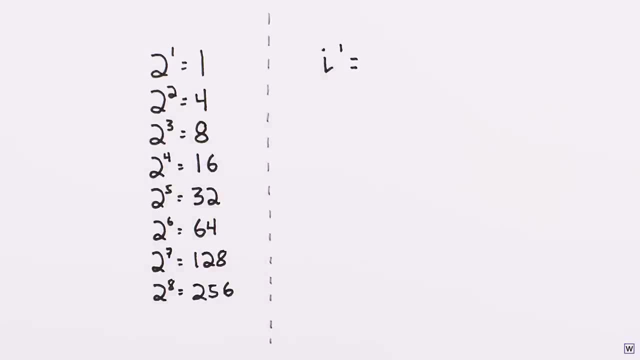 higher powers. it doesn't get bigger, as other numbers would. We know i squared is negative one from the definition and if we keep multiplying, i by itself, we see a pattern that repeats every four multiplications, over and over, and over and over. Hold on to. 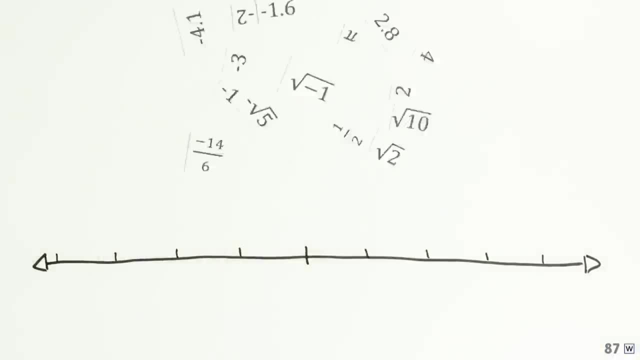 that fact for 90 seconds. Let's return to our friend, the number line. Remember that all the numbers we know about show up here, except imaginary numbers, They are nowhere to be found. If we think back to our original problem with the roots of negative numbers, 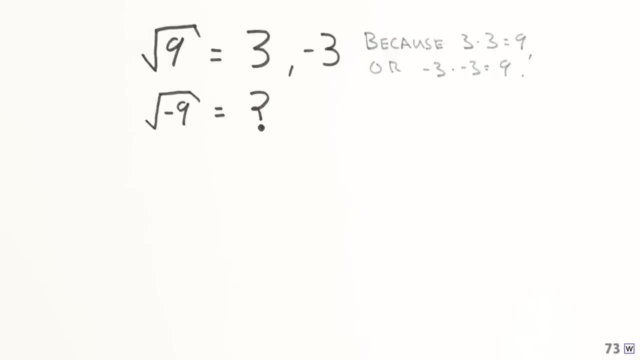 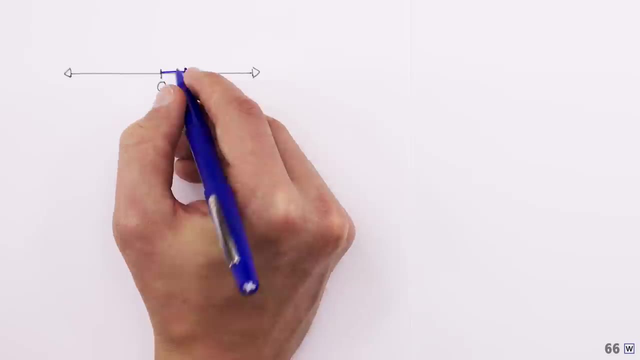 we can visualize this using the number line. Remember, the issue we had was finding a number that, when multiplied by itself, would yield a negative. To see this more clearly, we'll use arrows instead of dots to indicate numbers. Multiplying a positive by itself, maintains. 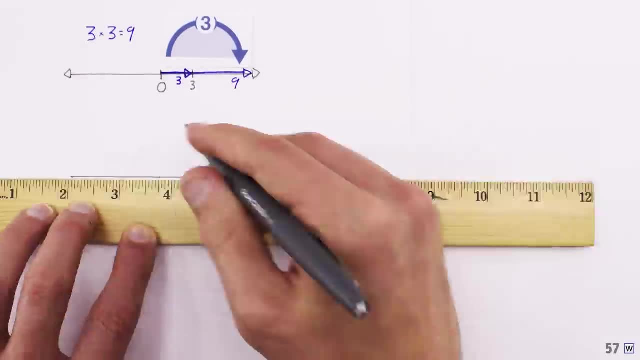 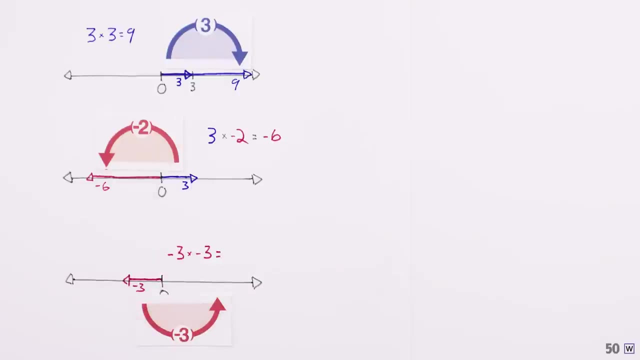 direction. on the number line It stays positive. If we multiply by a negative, we flip directions or rotate 180 degrees. Squaring a negative lands us in the positive numbers because we start on the left side with our first negative and rotate 180 degrees when we multiply by. 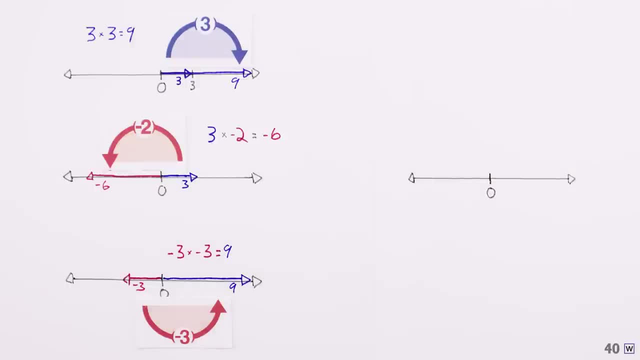 the second negative. So there's no way to land on a negative number when squaring, A positive squared results in a positive and a negative squared results in a positive. So we can't just use arrows instead of dots to indicate numbers Multiplying a positive. 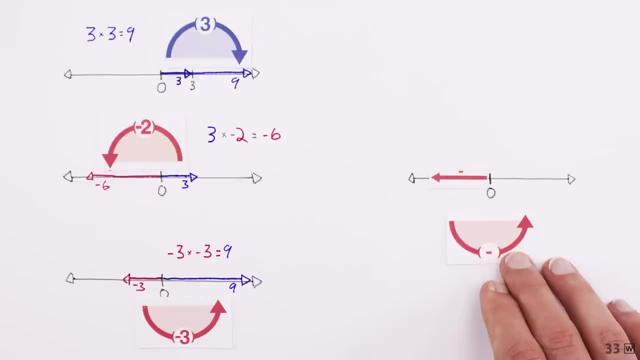 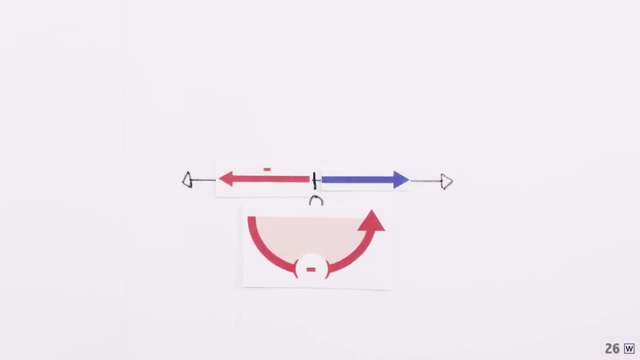 and a negative squared requires starting in the negative territory, and when we multiply by the other negative, we arrive back in the positive numbers. So what we need is something in the middle, A number that, when we multiply by it, only rotates 90 degrees, not 180 degrees as negatives do. 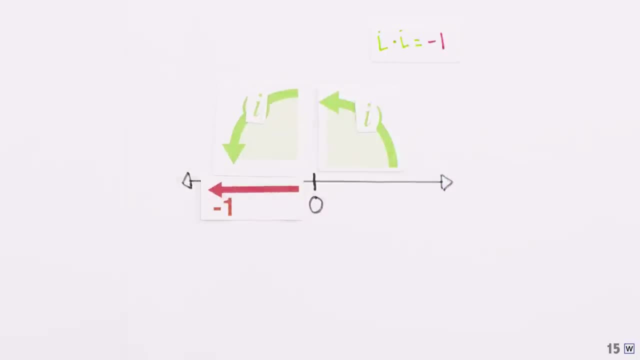 This is exactly what imaginary numbers do. i squared is negative 1, meaning that the first i puts us 90 degrees from the positive real numbers and multiplying by i rotates us 90 degrees further. exactly the same as the first i. So what we need is something. 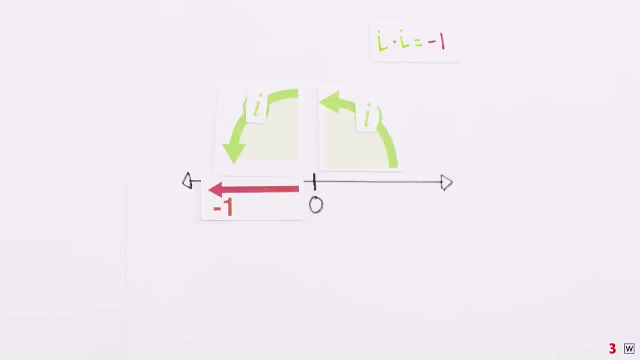 in the middle a number that, when we multiply by it, only rotates 90 degrees, not 180 degrees, not 1 centiaionths, because that means that the numberлю is in the vertical lower minded area in our strange number relationships. 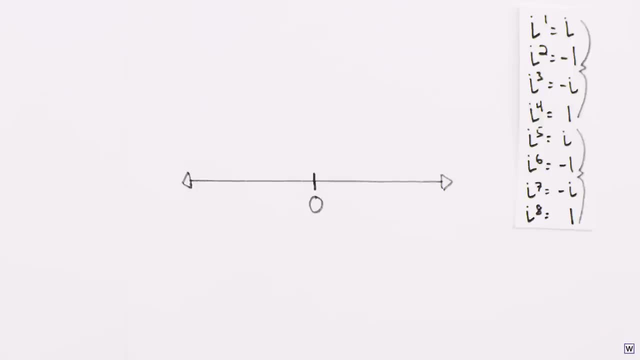 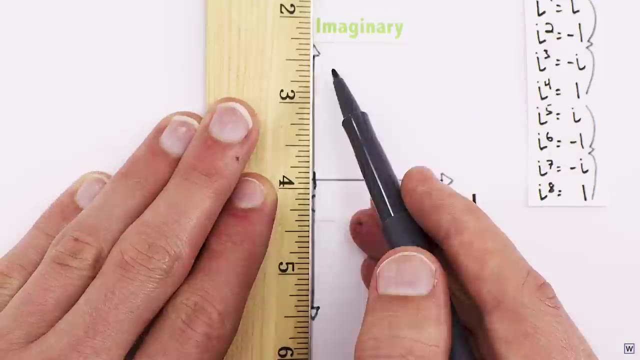 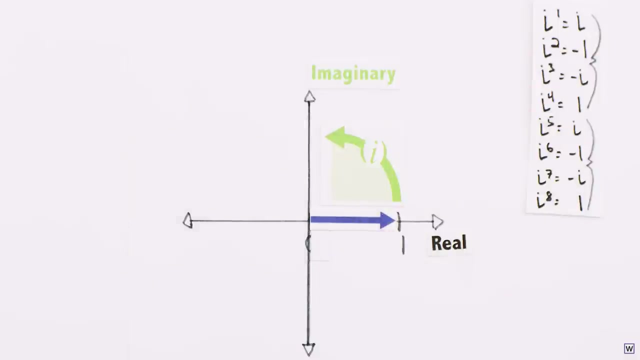 Going back into that factor you were hanging onto, Since multiplying by i corresponds to one 90 degree rotation. if we place our imaginary axis at a right angle to our number line, our algebra will perfectly fit with our geometry. If we start with the real number 1, and multiply by i, algebraically we get i, which geometrically 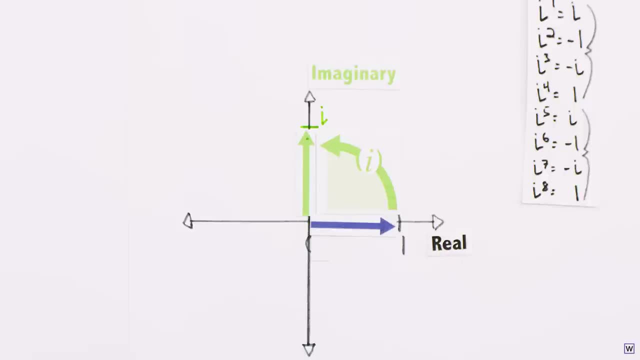 corresponds to the 90 degree rotation from i to 1.. Multiplying by i again is the first i, In other words that number two, can create a results in I squared, which by definition is minus 1 and again matches a 90 degree rotation. 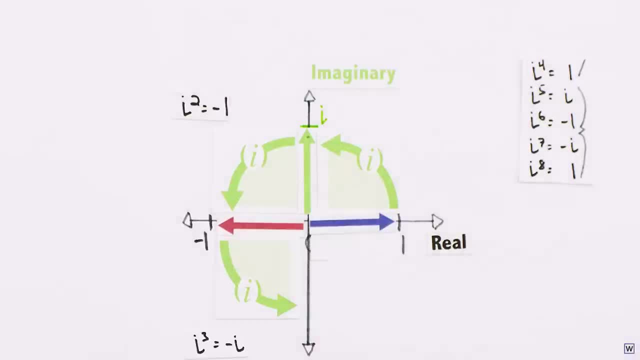 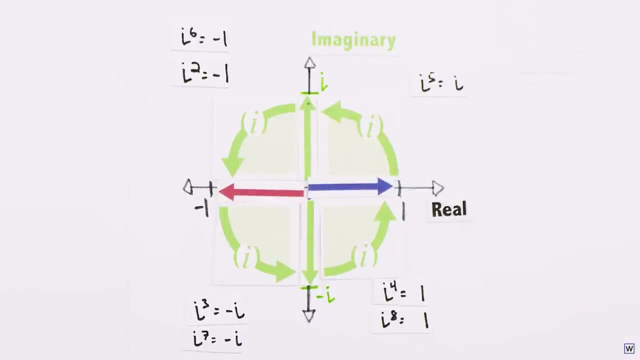 from I As we keep raising I to higher and higher powers. we keep rotating around with our values, repeating every fourth power, just as they did algebraically. So the big insight here is that imaginary numbers do not exist, apart from the real numbers. 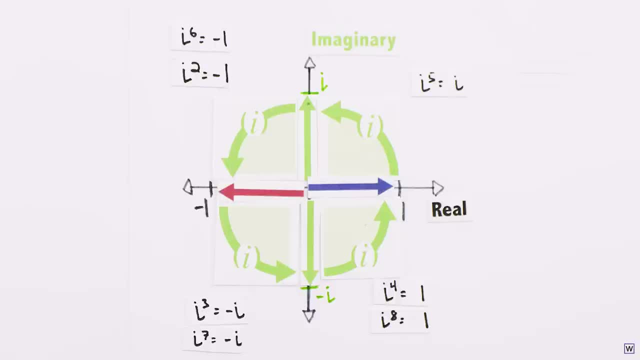 but right on top of them, hiding in a perpendicular dimension. This is the deeper meaning behind imaginary numbers. They aren't just some random extra number or hack. they are the natural extension of our number system from one dimension to two. Numbers are two-dimensional.